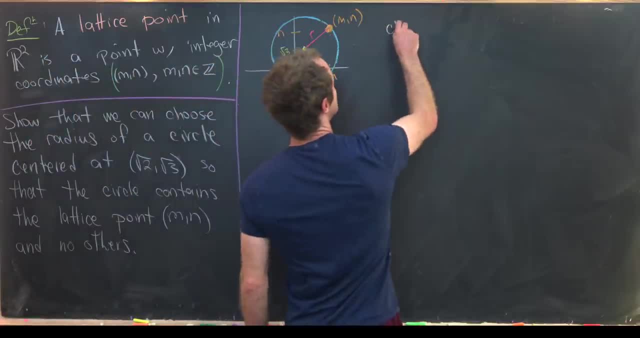 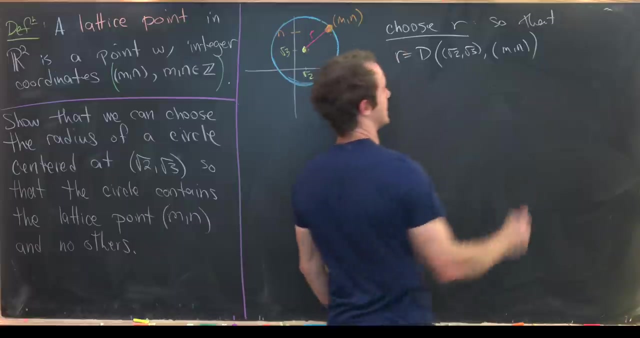 write down exactly what we would need. So let's choose r, so that r is equal to the distance from our point. square root of 2. square root of 3 to m? n. Notice, there wasn't any restriction on the radius over here. It didn't. 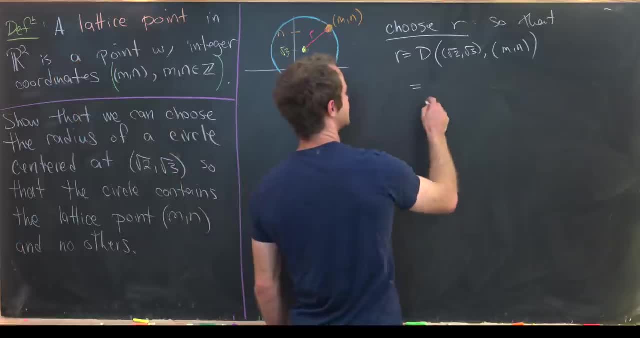 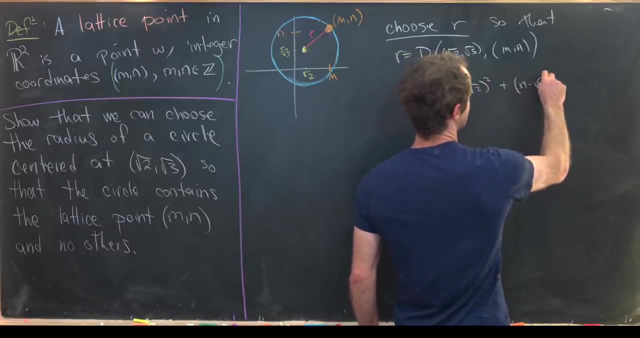 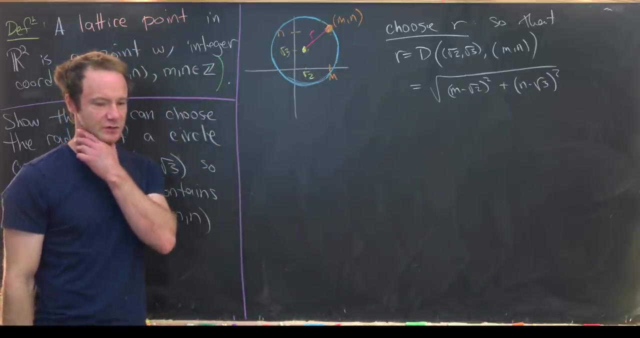 have to be an integer or even a rational number. That means that r is equal to the square root of m, minus the square root of 2 squared plus n, minus the distance from the origin in the x direction. So that's what we're choosing for our radius. Okay, so that wasn't too hard. We proved that. 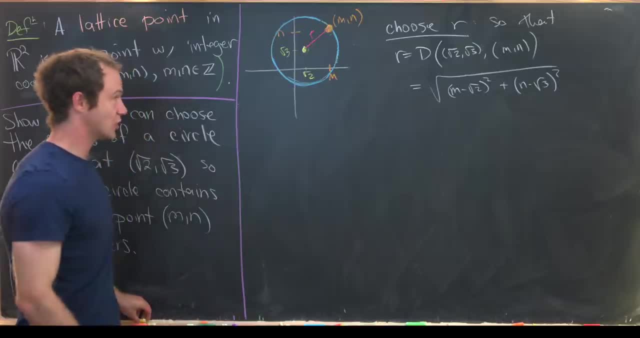 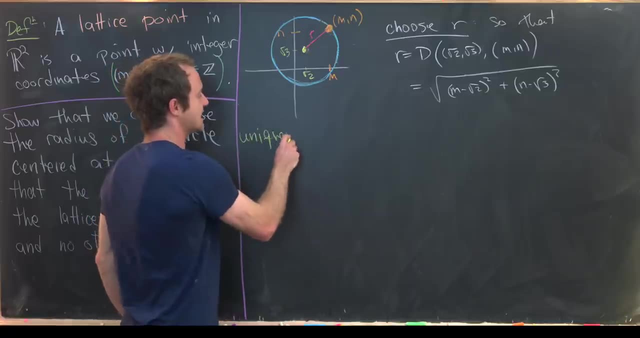 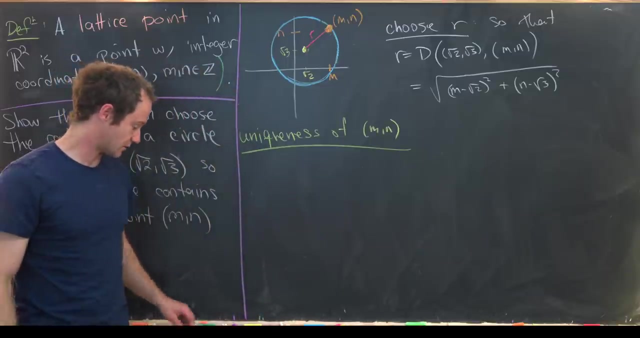 there exists a radius, so that our circle contains this lattice point m n. Now, next, we want to show something about the uniqueness of our lattice point m n on this circle, And we'll do that by supposing that we've got another point: square root of 2, square root of 3, squared plus n, minus the. 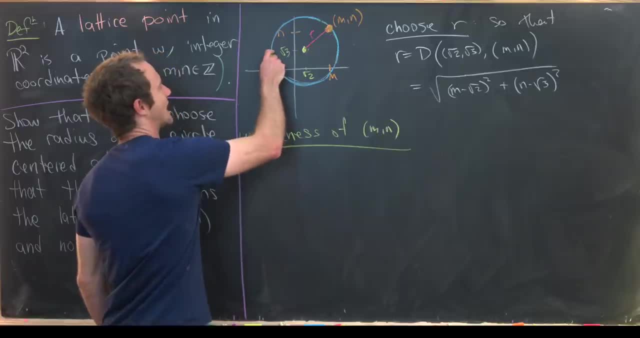 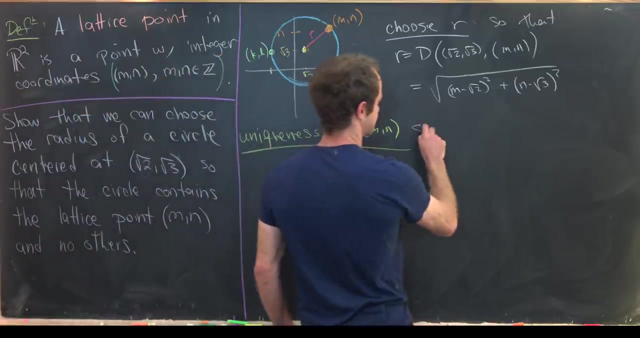 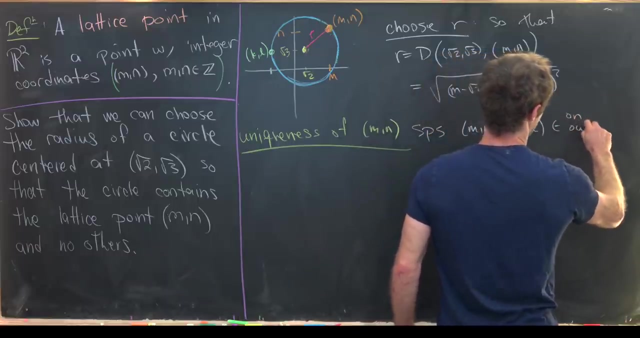 other lattice point on the circle. So maybe we'll put that lattice point over here. So notice, it's like a negative direction in the x axis and then some positive direction in the y axis. I'll call this kl. So let's suppose m, n and kl are both on our circle. I'll just write that to mean that. 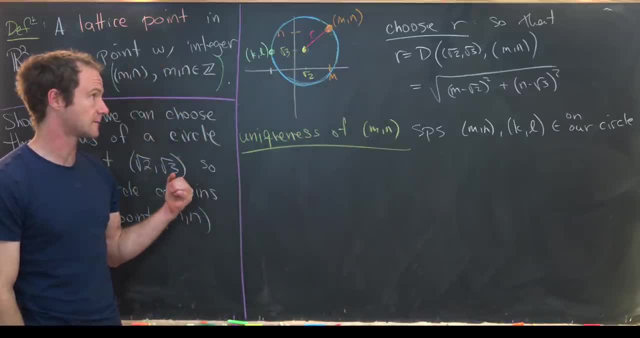 they're going to be on this blue circle of radius m n. So let's suppose that we've got a point, square root of 2, square root of 3, squared plus n, minus the square root of 3, squared plus n, minus the square root of 3, squared plus r, centered at root 2, root 3.. Okay, but that means they: 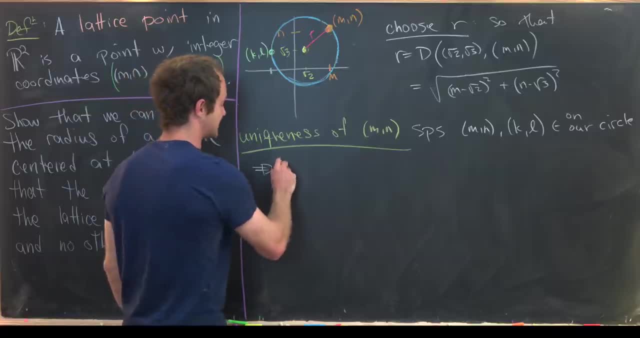 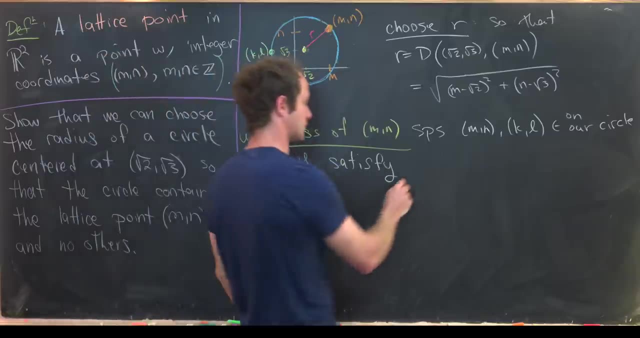 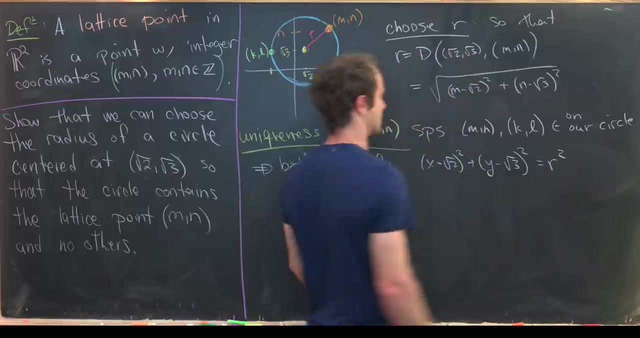 satisfy a certain equation. They both satisfy the standard equation for this type of circle, which is: x minus the square root of 2 squared, plus y minus the square root of 3 squared, equals r squared, which is essentially built out of this distance formula. Well, if they both satisfy that, 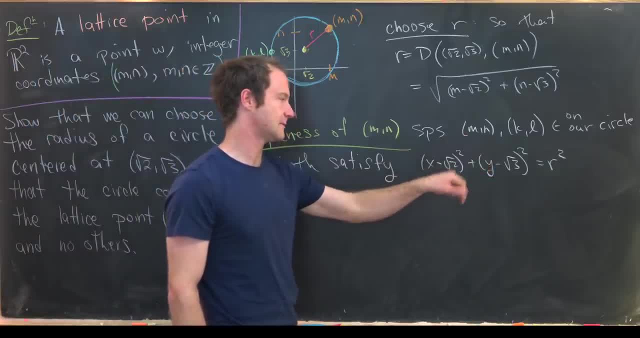 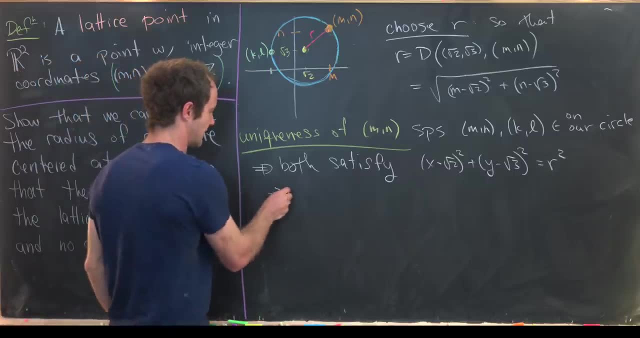 we can plug in m for x, n for y or k for x and k for y and we'll get r squared. But we can just set r squared equal to r squared and that'll give us the following equation: We have m minus. 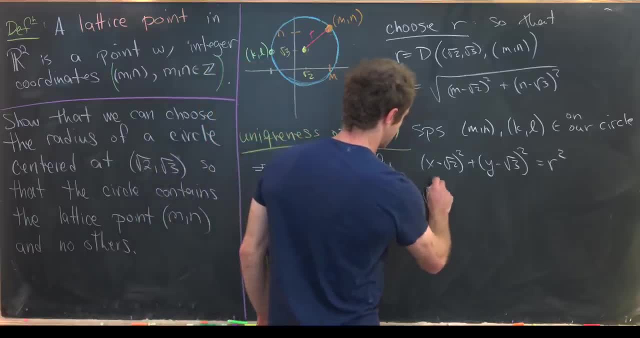 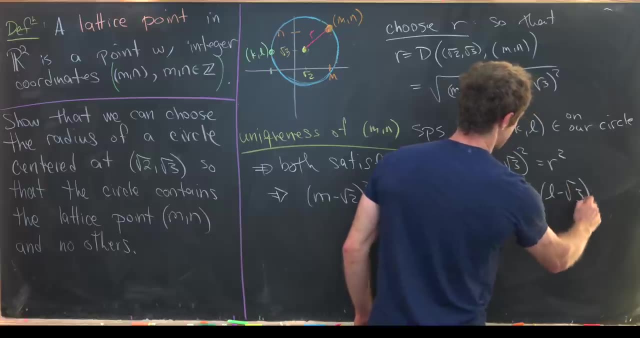 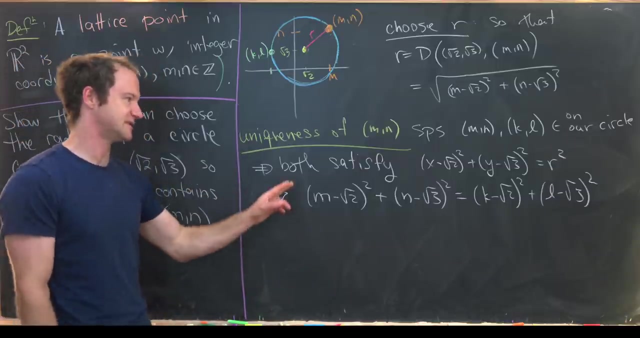 root 2 squared plus n minus root 3 squared equals k minus root 2 squared plus l minus root 3 squared. Okay, and then, since we're going for uniqueness here, we clearly want to show that m is equal to k and n is equal to l, but we're not quite there. 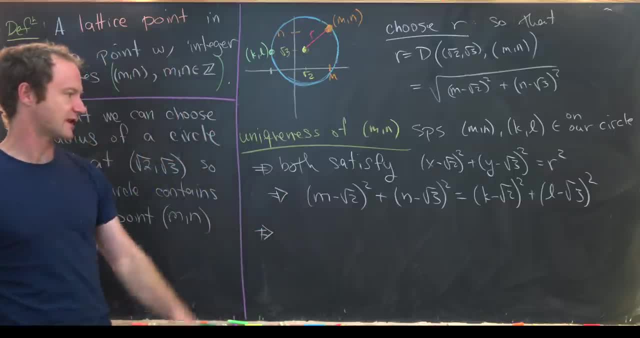 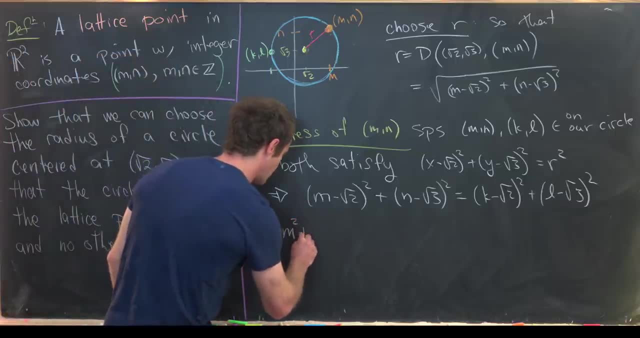 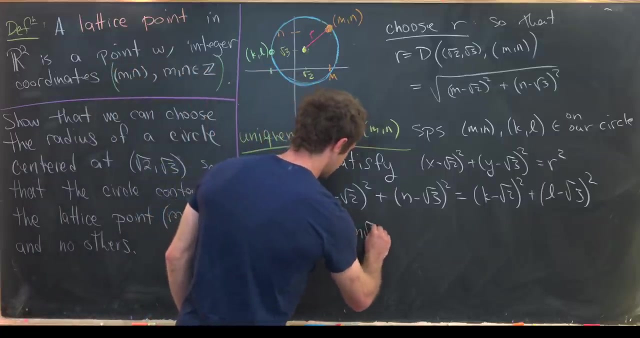 yet Okay. so where can we go from here? I'd probably like to multiply these out. I'm going to move some things around while I multiply them out, though, So I'll get m squared plus n squared, and then minus 2m times the square root of 2, and then minus 2n times the square root of 3. 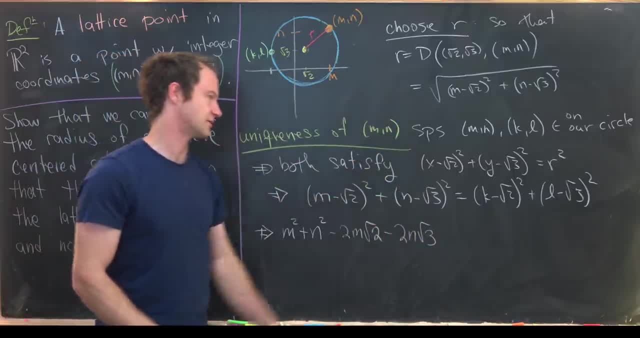 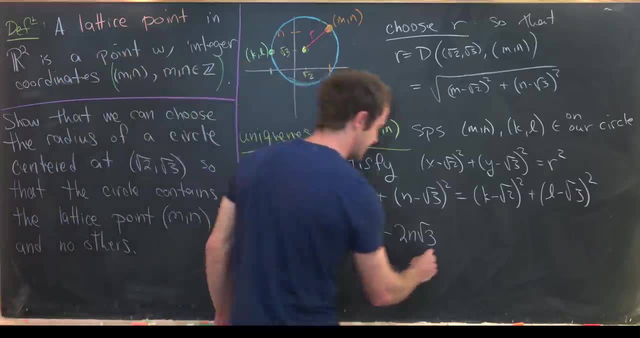 so that comes from the cross term here and the cross term here, And then we'll have root 2 squared, which is 2, root 3 squared, which is 3.. 2 plus 3 is 5.. So that's what we get if we multiply all. 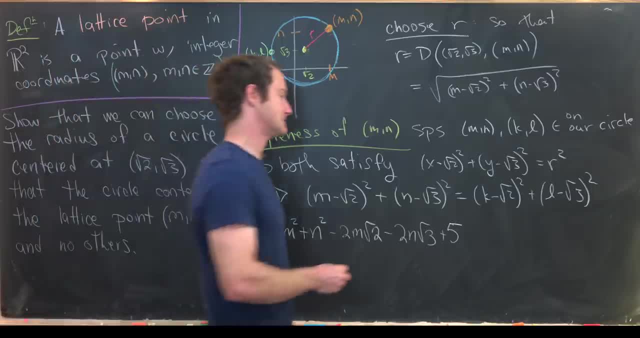 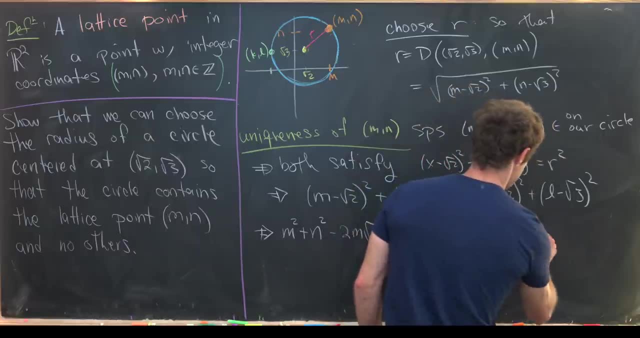 of this out and then move some things around. Okay, but now let's notice that this is going to be equal to k squared plus l squared minus 2 times k. times root 2 minus 2 times l. times root 3 plus 5.. 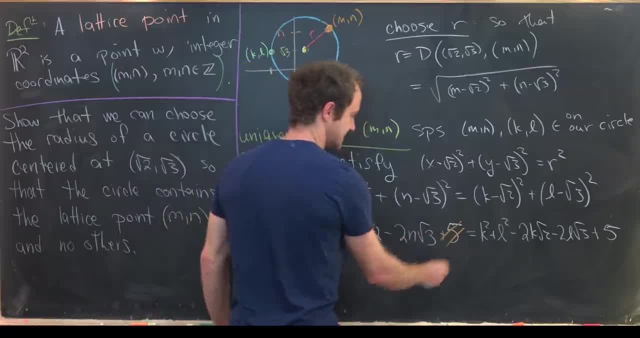 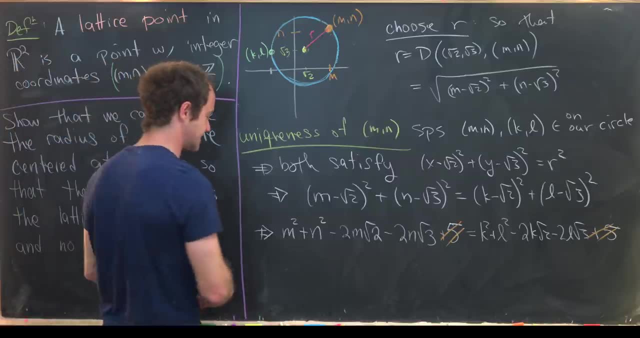 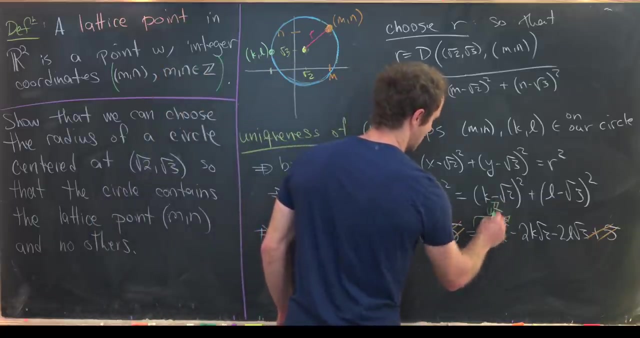 Now we can do a bit of simplification, So notice, I can take this 5 and subtract it from both sides, So that's good to see. Another thing that's nice to notice is that m squared plus n? squared is most definitely an integer, and k squared plus l squared is also most definitely an integer. 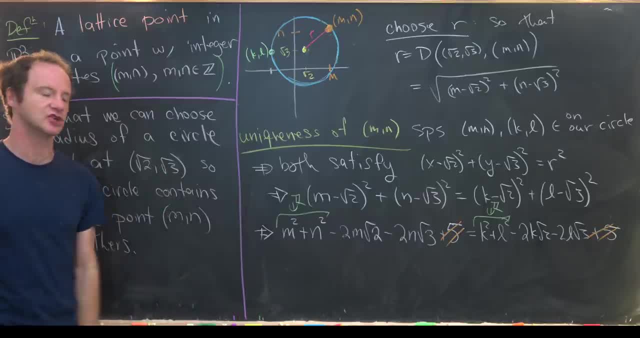 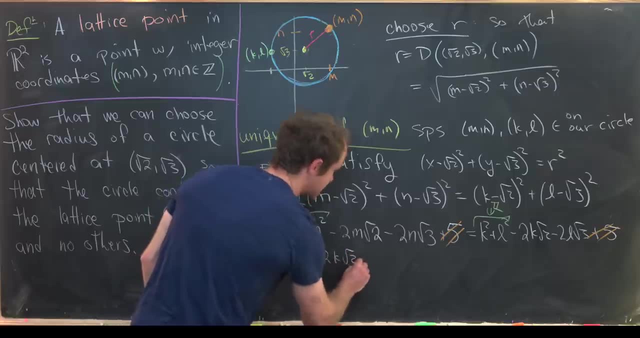 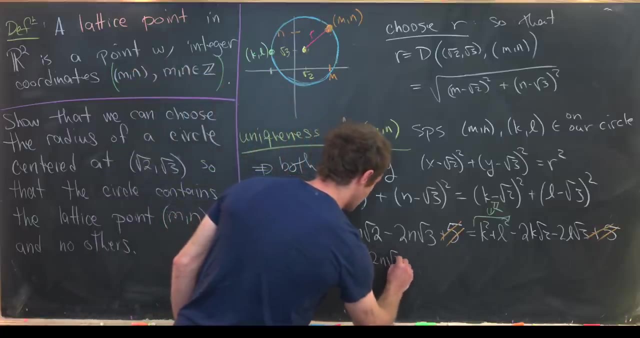 So maybe it'll be useful to move everything that's an integer to one side of the equation. That'll give me 2m root 2 minus 2k If I move this m over there and then plus 2n root 3 minus 2l root 3,. 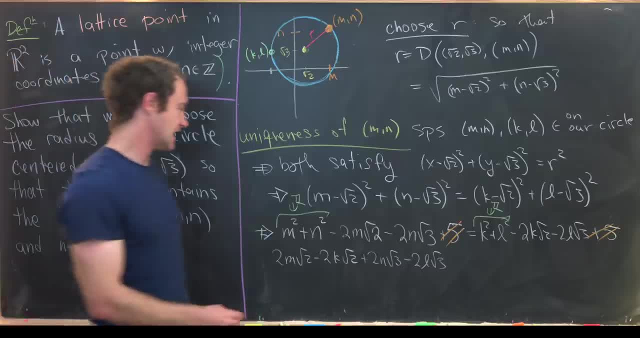 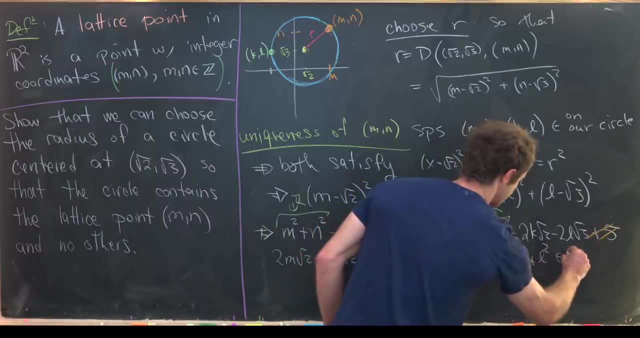 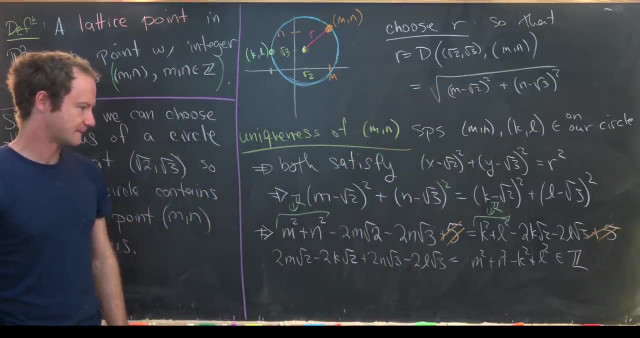 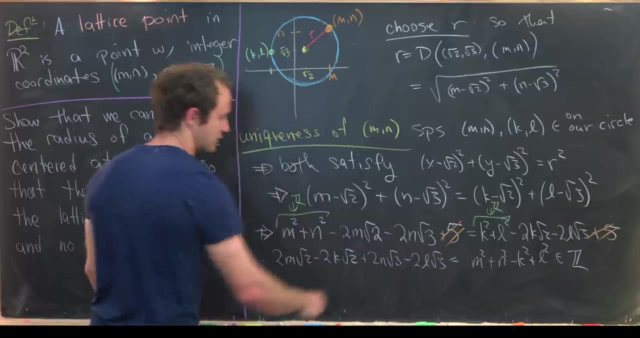 if I move my n part over there, equals m squared plus n squared, minus k squared plus l squared, which is an integer. Okay, nice, But now notice, we can do some factorization over here, So maybe we can factor it. We can take 2 out of everything and a root 2 out of these first two terms and a root 3 out of these. 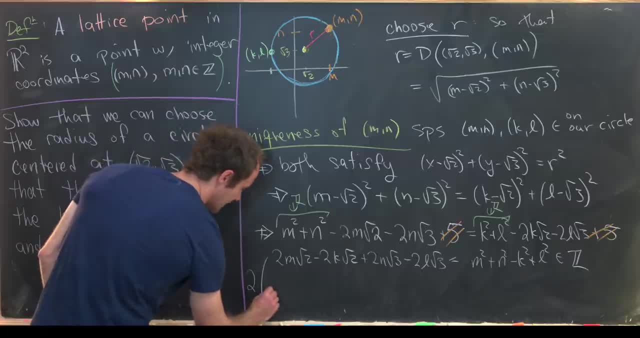 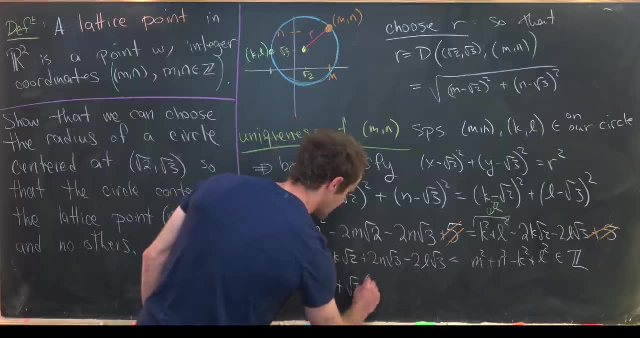 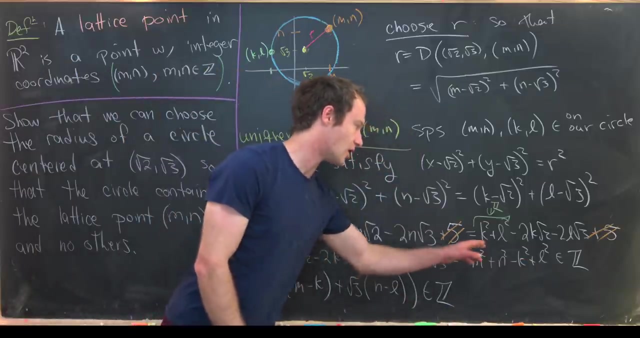 second two terms. So that gives us 2 times the quantity. the square root of 2 times m minus k plus the square root of 3 times n minus l must be an integer. Notice, we don't care what this is anymore. All that we care is that it is an integer, and I was missing a l or a minus sign there. 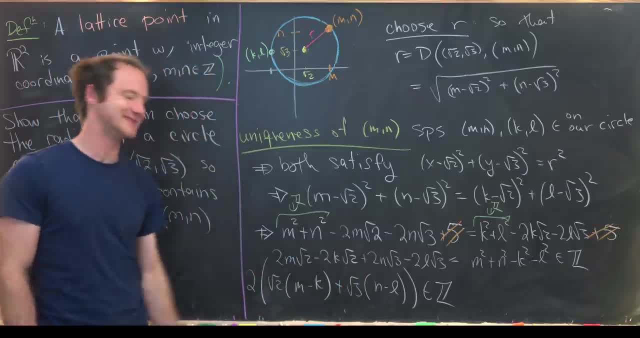 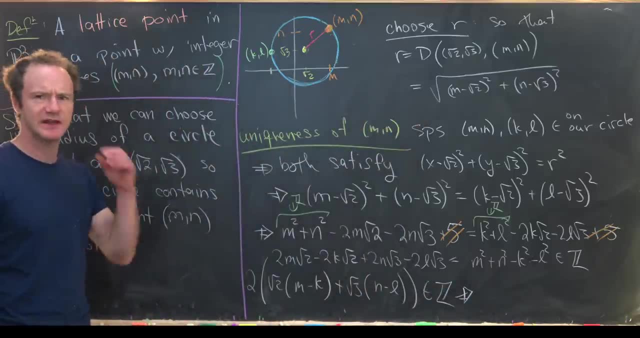 But notice that we don't care what this is anymore. We don't care what this is anymore. Now let's notice: if 2 times this object is an integer, that means this object on the inside is a rational number. We don't know that it's an integer. It could be an integer over 2.. 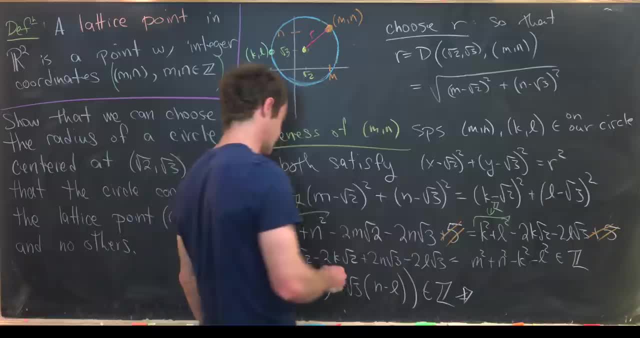 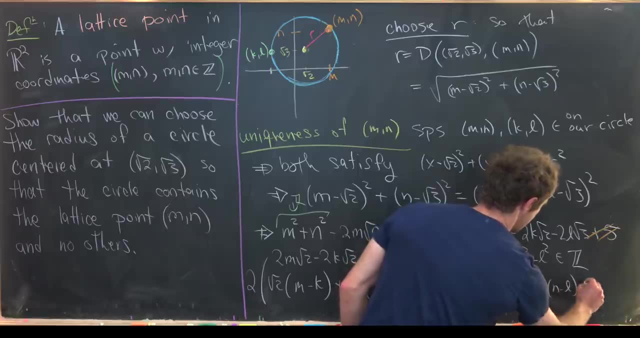 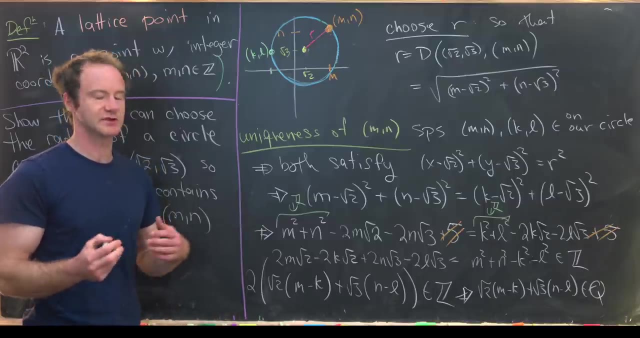 We'll just like keep it a little bit more general and say that it's a rational number. So we have the square root of 2 times m minus k, plus the square root of 3 times n minus l must be a rational number. Now, if you know anything about field extensions of the rational numbers, 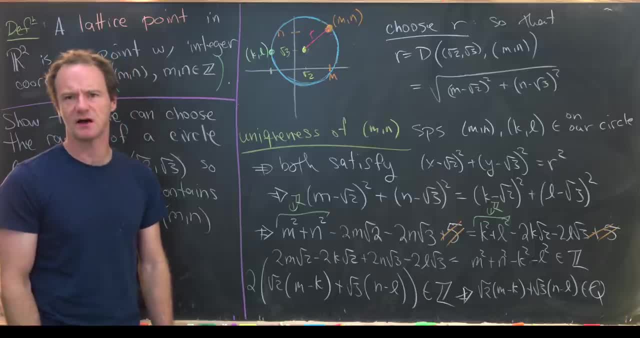 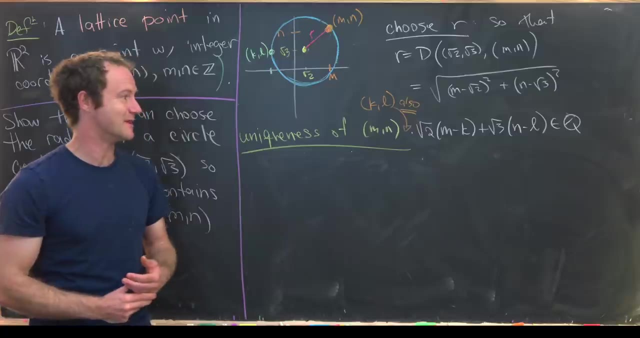 you immediately know that m is equal to k and n is equal to l. But let's assume that we don't have that knowledge and work through the details, Okay, so let's maybe get rid of some of this and then move on to the end. So we're almost done proving the uniqueness of our lattice point m. 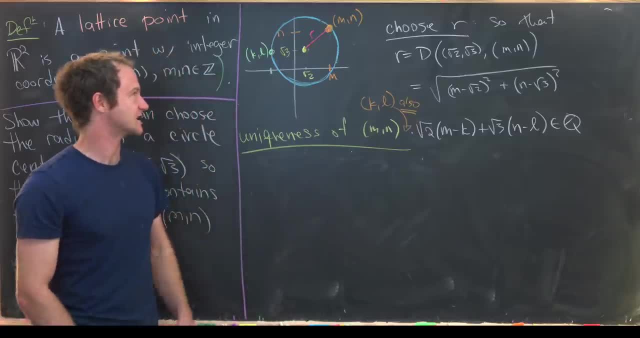 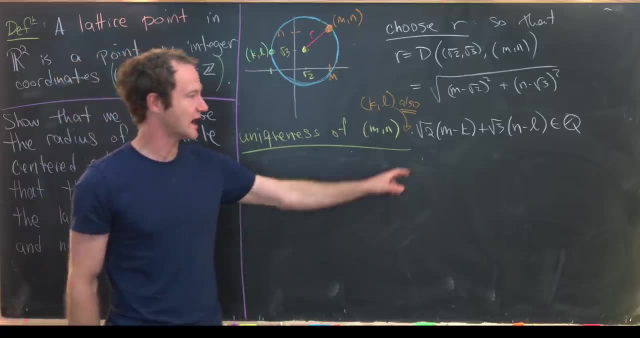 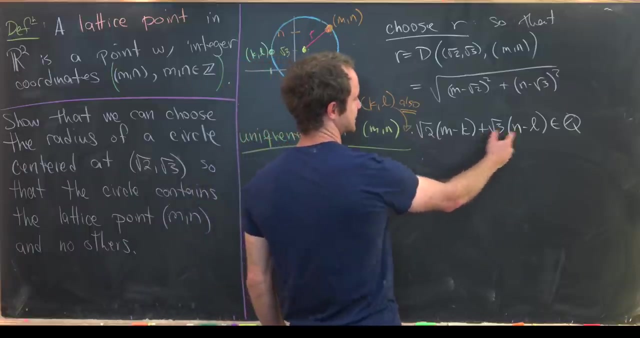 n. So we assume that k? l was another lattice point, kind of like this picture up here, And we want to show that this implies that k l is equal to m? n. We got it down to the following spot where we have the square root of 2 times m minus k plus the square root of 3 times n minus l. 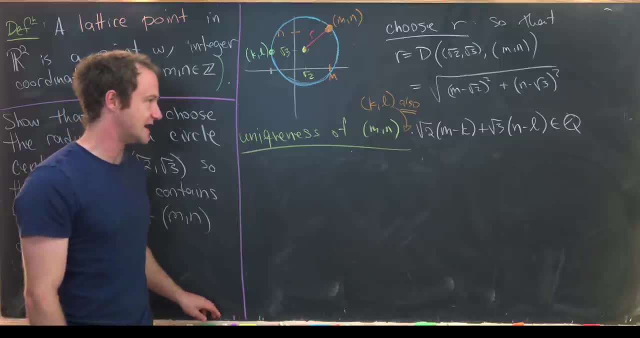 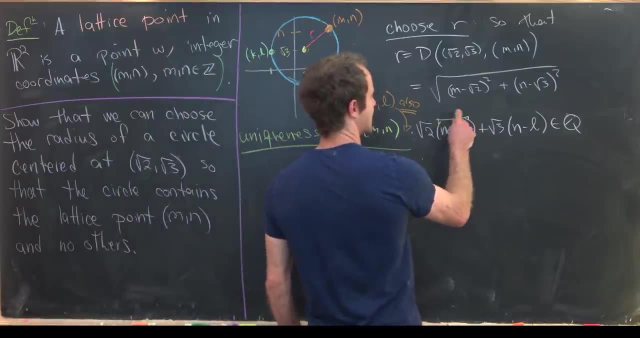 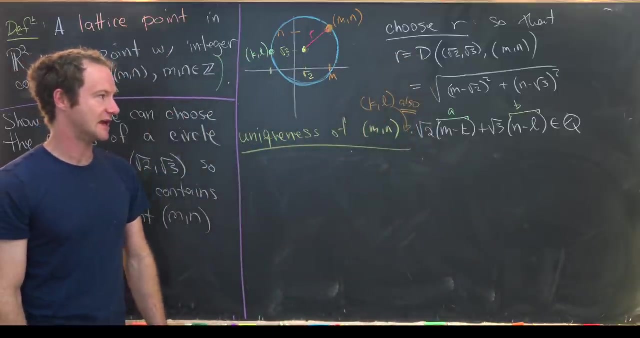 is a rational number. Okay. so from here I want to introduce a little bit of notation that's going to provide a simplifying effect. Maybe I'll call this guy right here equal to a and this guy right here equal to b. So in other words, we have: m minus k is a and n minus l is equal to b. 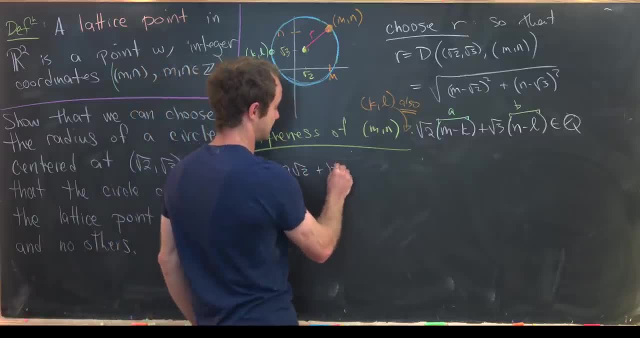 Now rewriting this, we have a times the square root of 2 times m minus k, plus the square root of 3 times n minus l is a rational number. square root of 2 plus b times the square root of 3 is a rational number. Now we can square that. We. 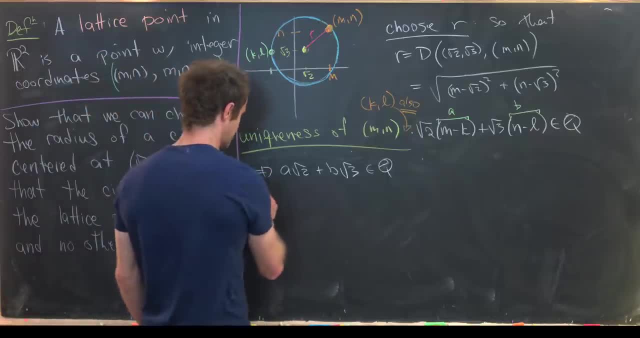 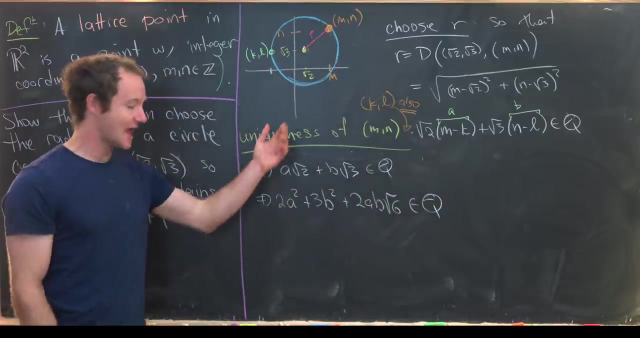 know that the square of any rational number is a rational number. So that's going to give us 2 times a squared plus 3 times b squared plus 2ab times. the square root of 6 must be a rational number. Well, since a and b are integers, we know that this whole thing over here is an integer. 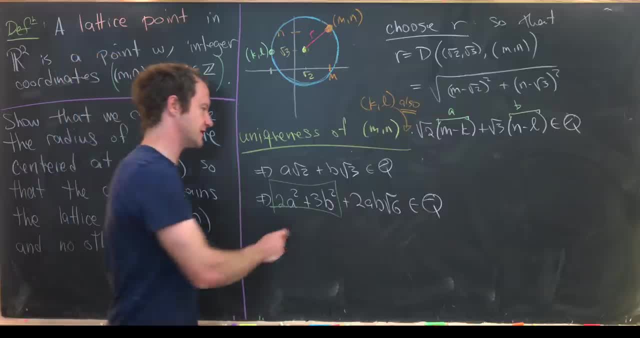 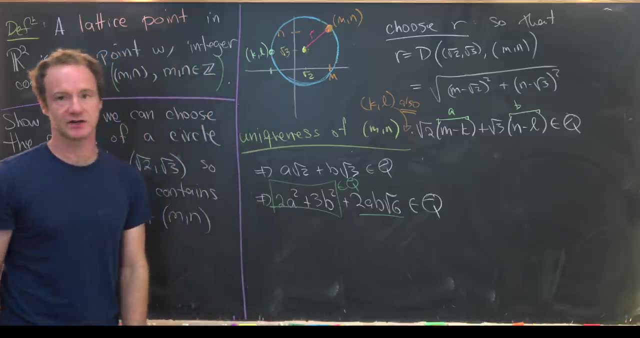 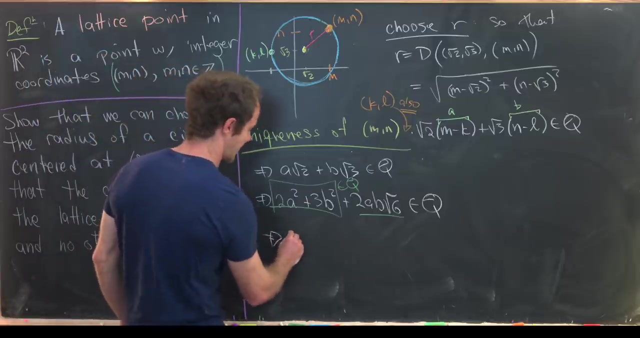 But integers are a subset of the rational numbers. So this whole thing right here is a rational number, which means that this remaining bit must also be a rational number, because the rational numbers are closed under addition. So that tells us that we've got 2ab times the square. 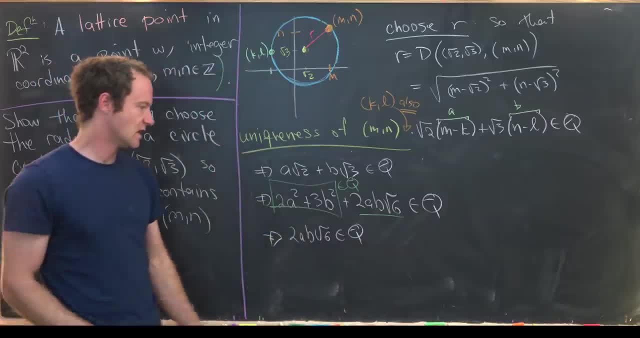 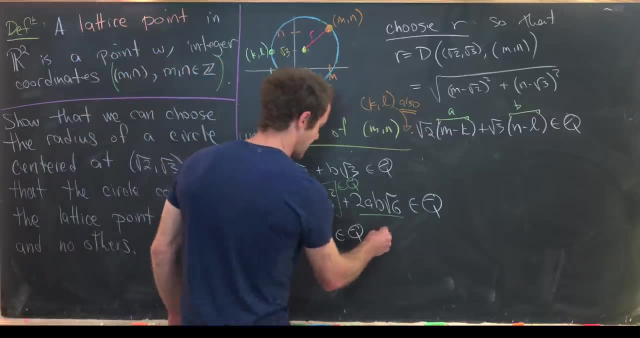 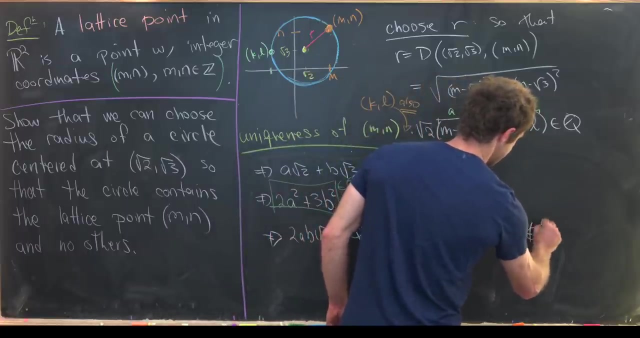 root of 6 is a rational number. But we know that the square root of 6 is not a rational number and a and b are integers. So we know that the square root of 6 is a rational number. So that means that a times b is equal to 0.. And let's see. that's because the square root of 6 is. 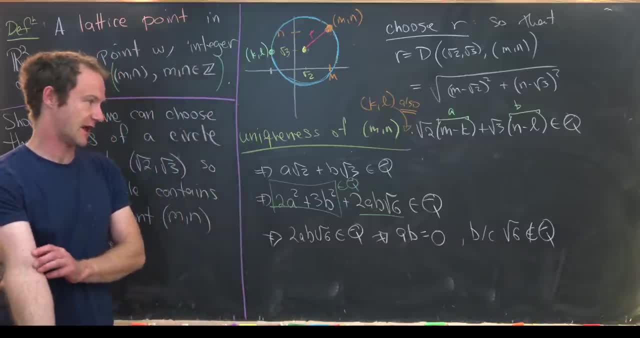 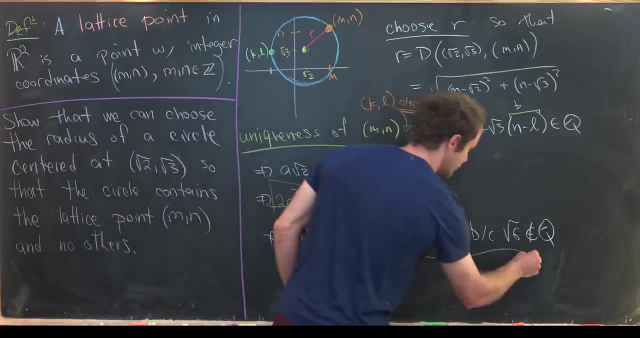 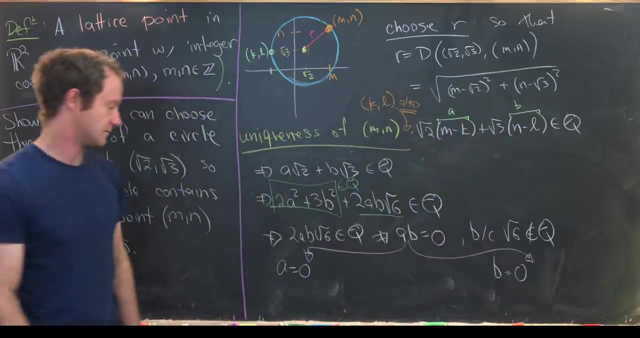 not rational. So pretty easy proof for that. I'll let you guys look for that if you need to. Okay, so if a times b is equal to 0, that actually splits off into two cases. That splits into the case a is equal to 0 or the case b is equal to 0. So notice, if a is equal to 0, m is equal to. 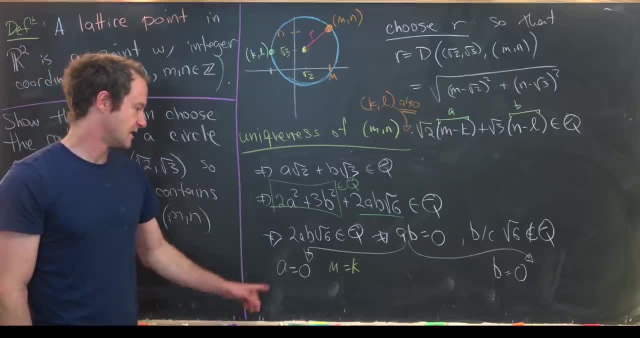 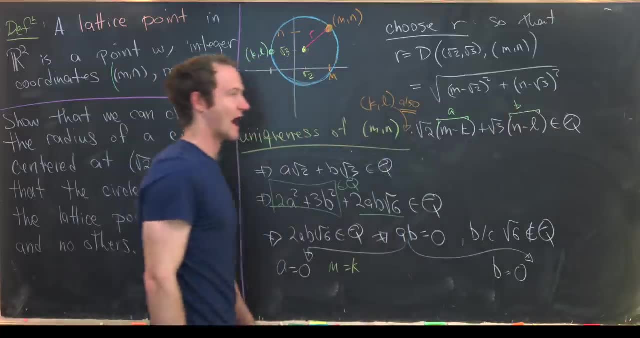 k. So that's good to keep in mind. But if a is equal to 0, back up here we see that the square root of 3 times b is a rational number. The square root of 3 is irrational. That means b has to be. 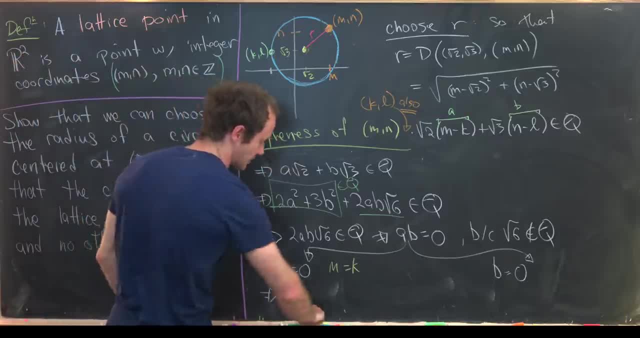 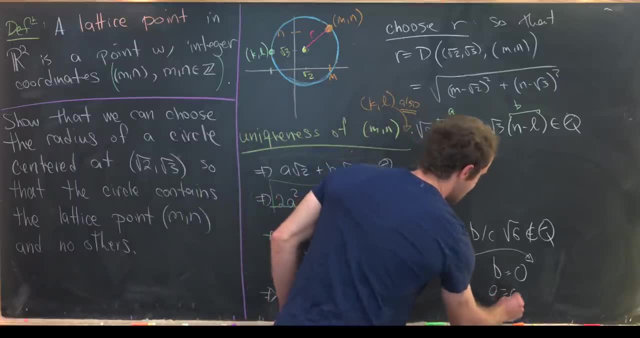 0.. So here we have: if a is 0, then b is 0. And thus n equals l, And then similarly over here: if b is 0, then a is also 0. That's because the square root of 2 is: 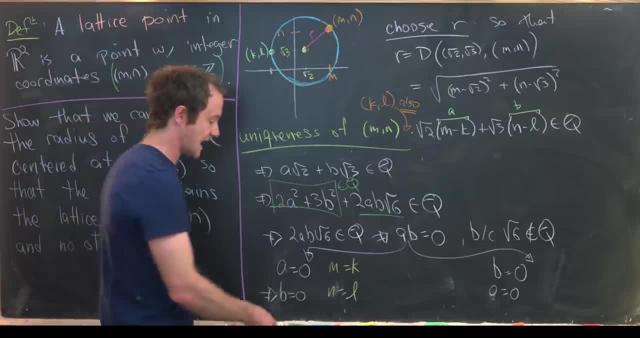 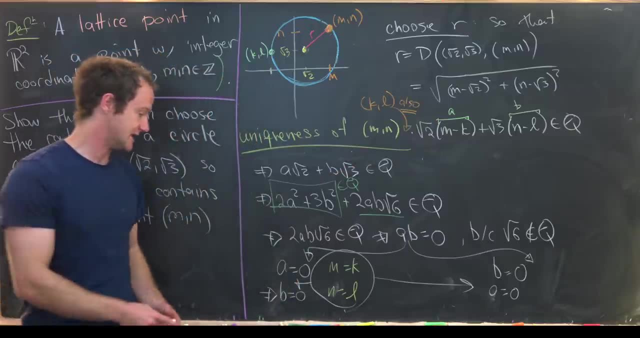 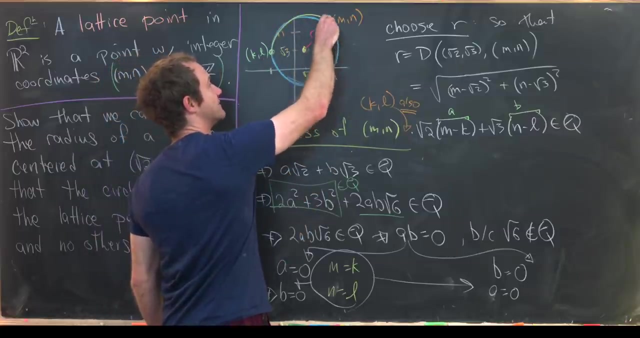 irrational, And so that means that m equals k and n equals l in both of these cases. But that means that our lattice point mn is in fact the same thing as our lattice point kl, So that means this guy can't live over here. It's in fact coincident with our original lattice point.